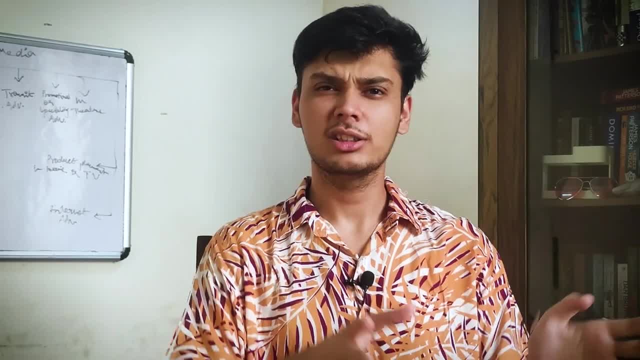 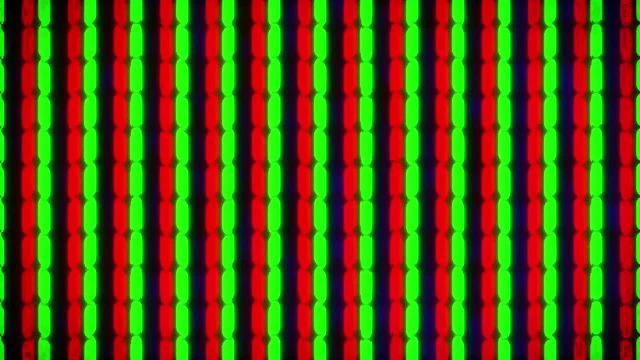 they are on your screen. and your screen is made up of pixels- red, green and blue pixels. So you are not looking at yellow, you are looking at a combination of red and green pixels. Inside your eyes, there are specialized cone cells that are sensitive to different. 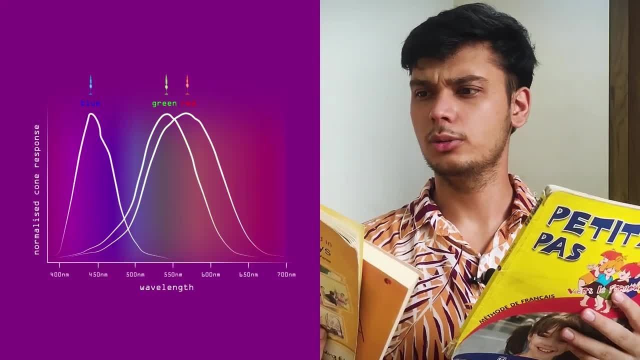 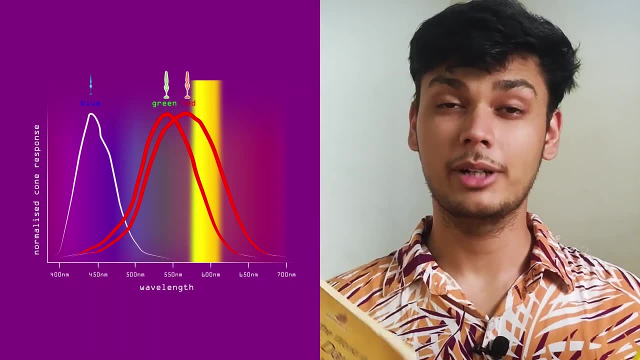 wavelengths of light. When actual real yellow light, reflected from these books about 580 nanometers, is hitting my eyes, some of my red and some of my green cone cells are activated. So my brain says, oh, this must mean that light hitting the eye is somewhere between: 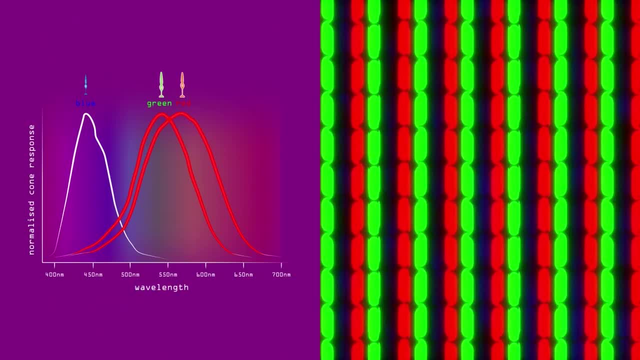 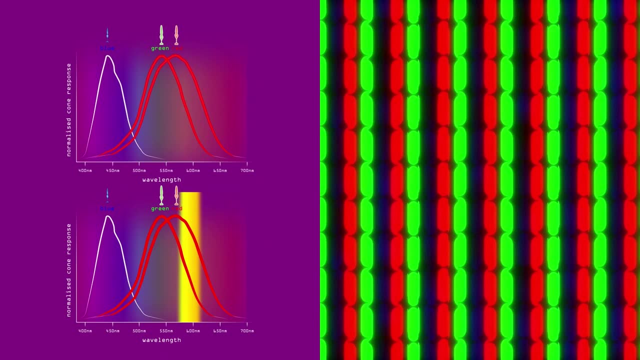 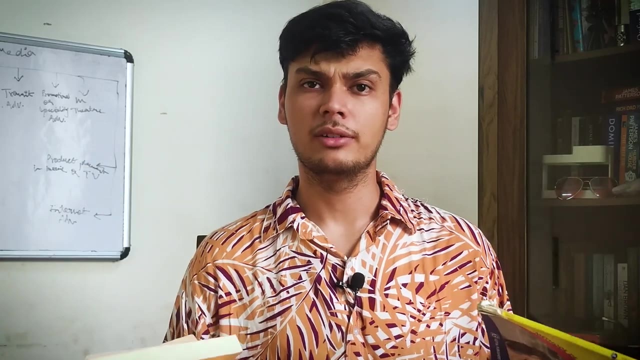 red and green wavelengths, So I see yellow. The pixels on your screen activate your cone cells in the same way, but your brain has no way of distinguishing between this and this, So it shows you yellow as well. Wait, hold on. Why are we talking about yellow? Let's talk about purple and violet. 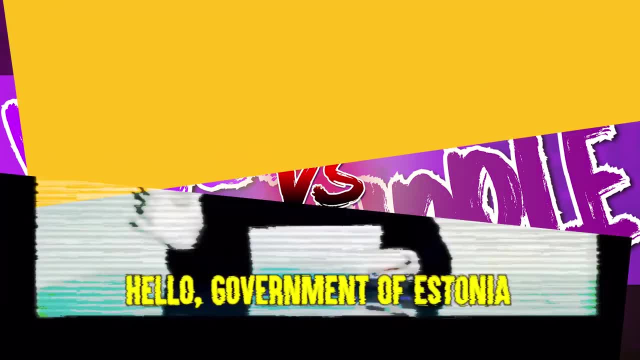 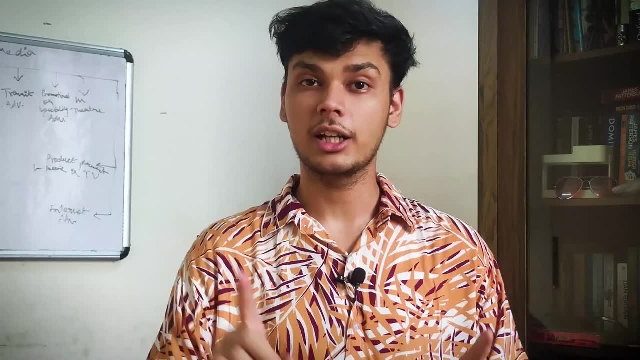 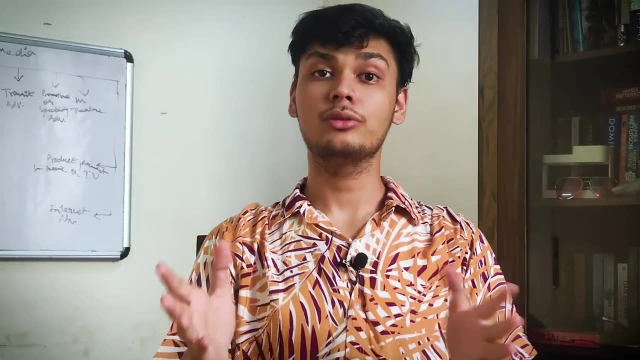 Hello, give them the best, donia. Wavelength of violet light is about 380 to 450 nanometers And wavelength of purple light is…. Haha, You pussgut. Purple light does not exist. Purple light has no wavelength. In fact, none of the combinations. 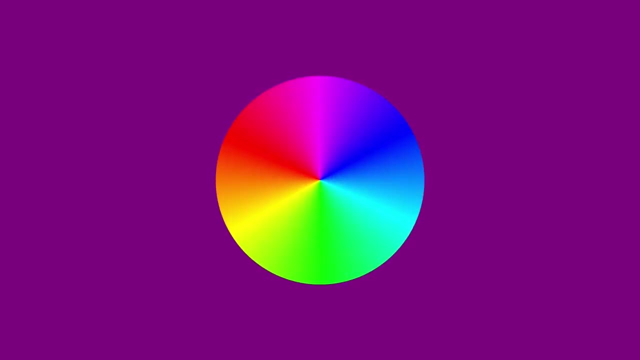 of red and blue have a wavelength. Every part of the color wheel, from purple to pink to magenta to fuchsia, have no wavelength. No light. Red and blue colors never meet in the rainbow or the electromagnetic spectrum, So there is no natural light that can activate only the red and blue cone cells in your eyes. 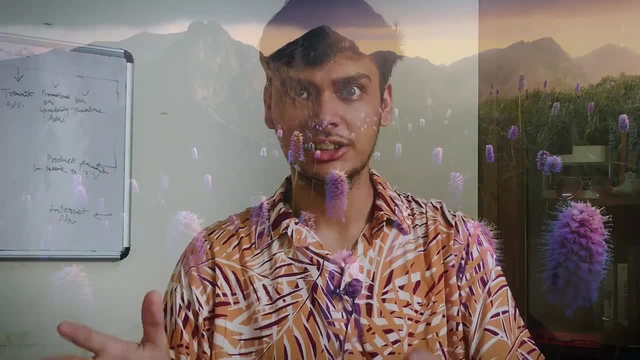 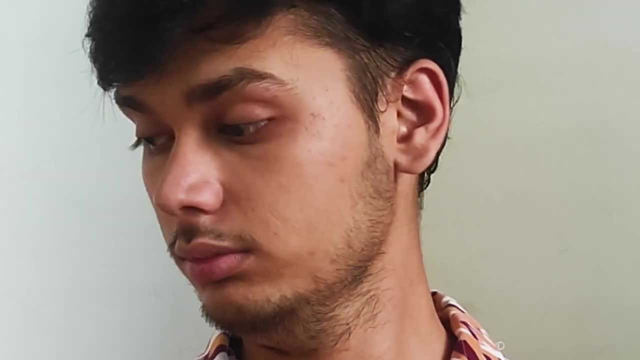 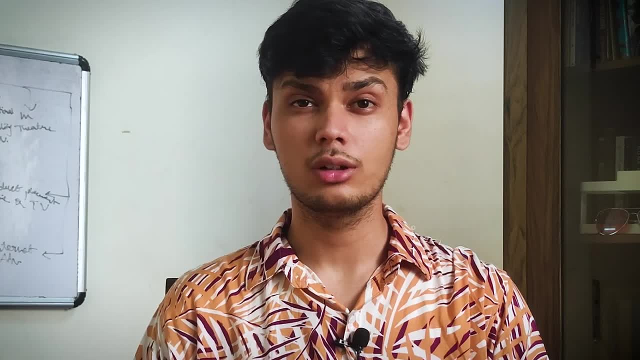 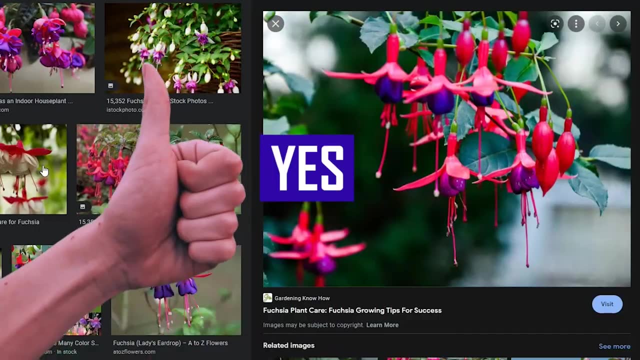 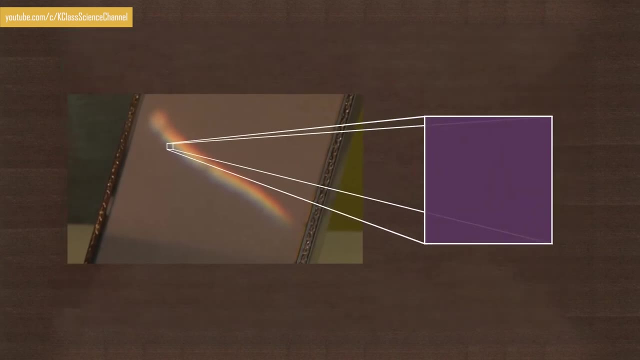 Isn't this unnatural? Isn't this natural? Isn't this natural? And look at the electromagnetic spectrum itself. You can call this violet or whatever, but I can clearly see a combination of red and blue. I'll call that purple. I'll check. 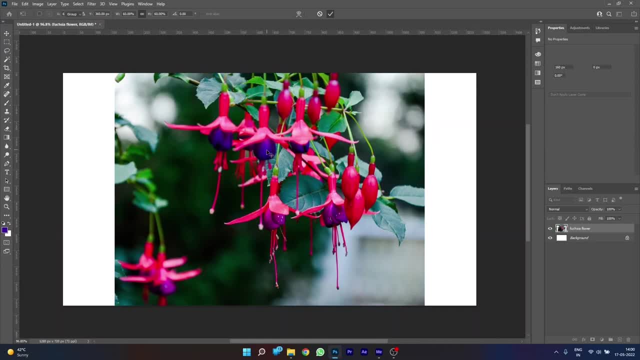 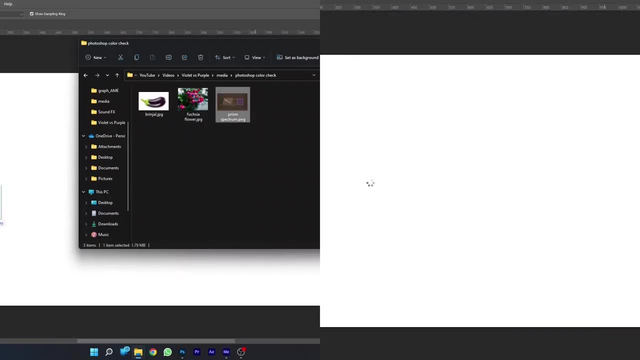 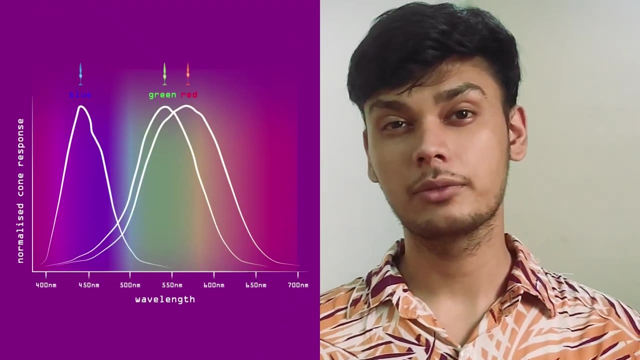 Let's bring all of these images into photoshop and check their color codes And we'll re-, And we'll rea-. Wait, it is a combination of red and blue. It is purple. What is happening? We call the light from 380 to 450 nanometers violet. 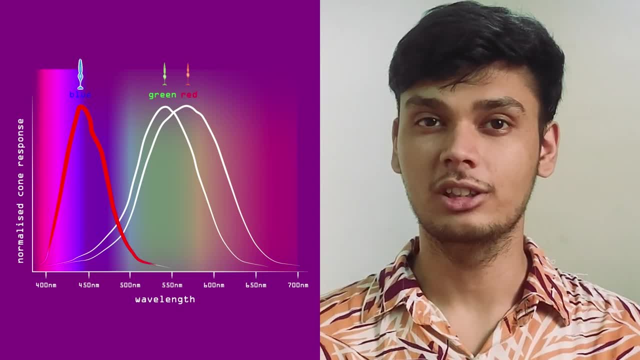 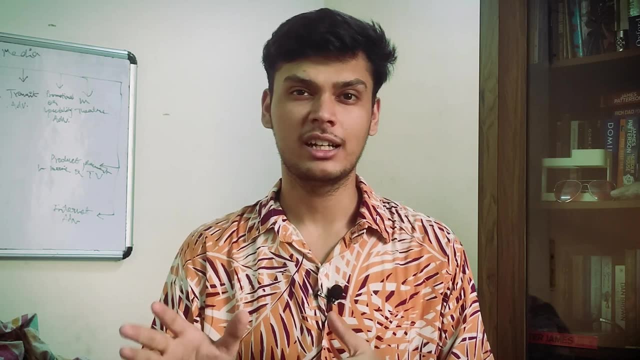 And it activates these cone cells, a part of blue cone cells. And this is where the confusion stems from. We've been calling the cone cells red, green and blue cone cells the entire time. Hence we think that whenever blue cone cells are activated, we see blue color. 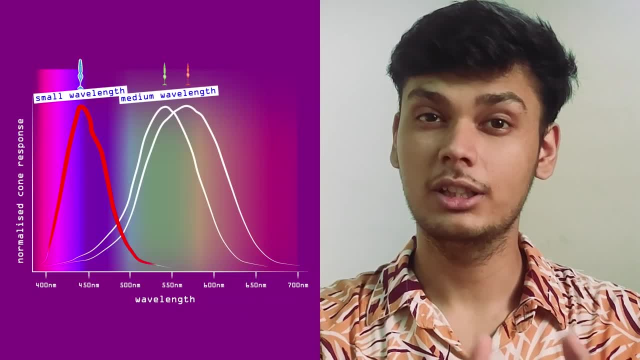 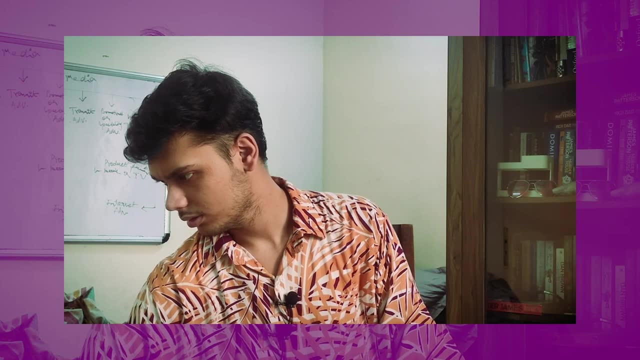 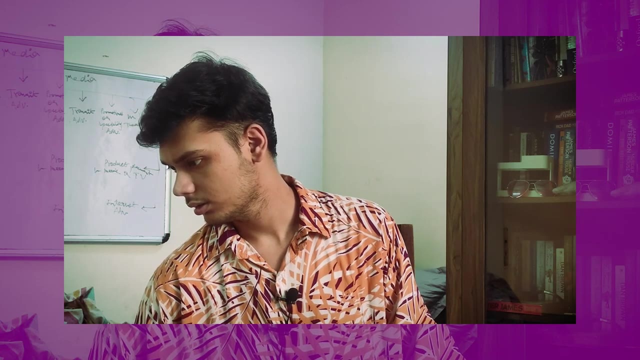 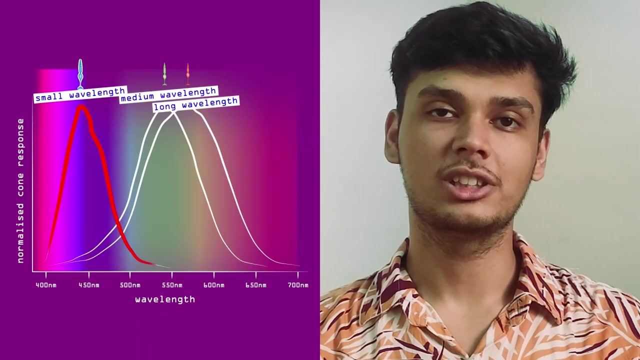 But it is much more appropriate to call them long wavelength, medium wavelength and short wavelength cone cells. Blue is long or short Blue versus red wavelength. Blue is a shorter wavelength, okay. Blue or short wavelength cone cells are also responsible for blue. 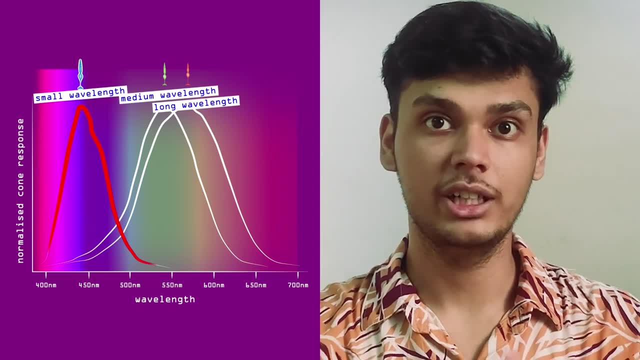 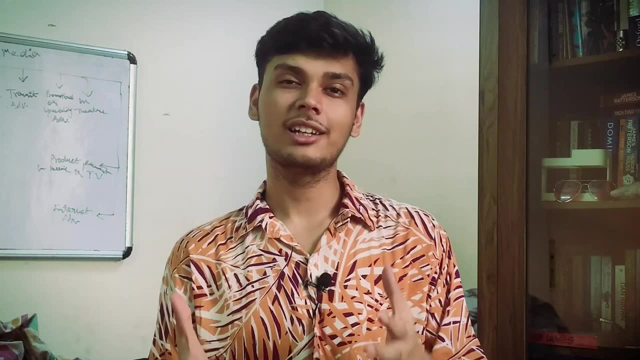 Blue is responsible for violet colors that we see, Colors in the range of 380 to 450 nanometers, So all of those naturally occurring purple things, Just violet. But we don't like thinking of violet as a separate color, like red and green and blue. 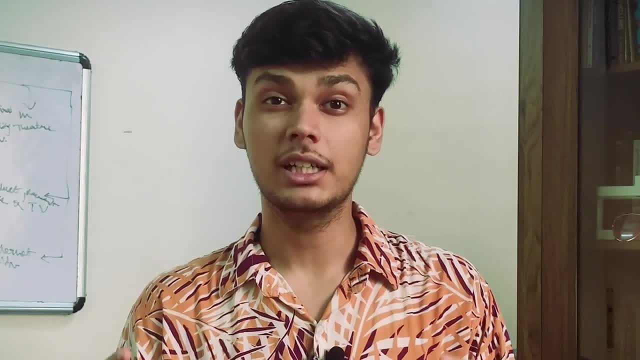 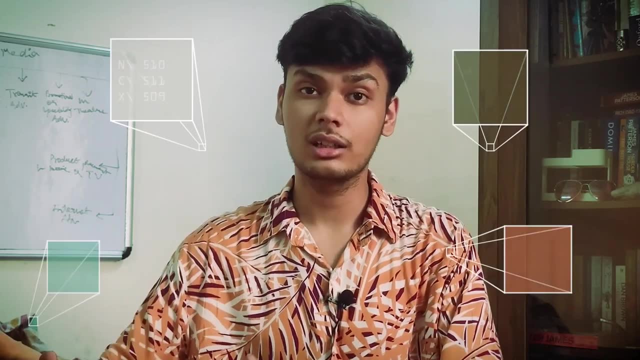 Because it doesn't fit the color wheel, And we as a society really like our color wheel. I mean, what's not to like about it? It makes it so much easier to think about colors. It reduces every color down to a three-dimensional value. 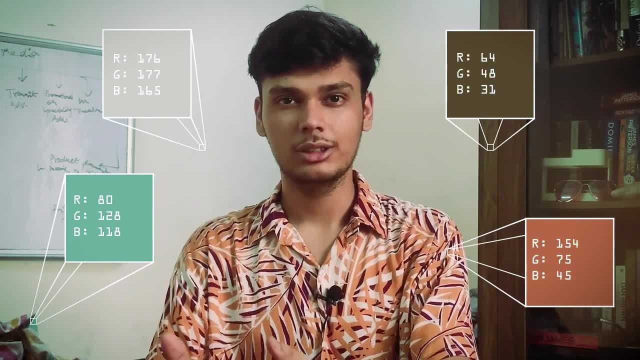 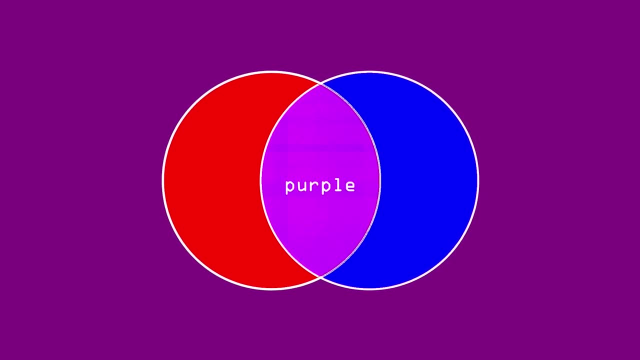 The amount of red, The amount of green And the amount of blue. The only problem is that it leaves no space for violet. The combination of red and blue makes purple Not violet. It's just that purple and violet despite being so dissimilar that one of them doesn't. 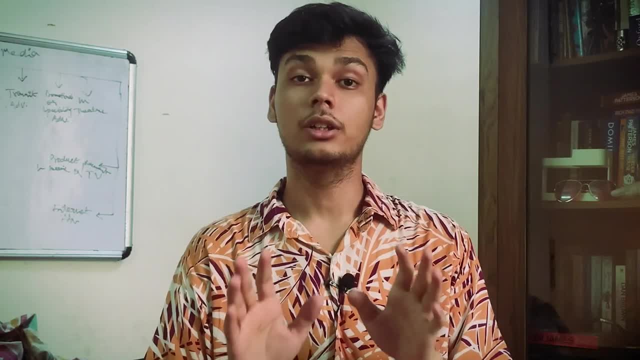 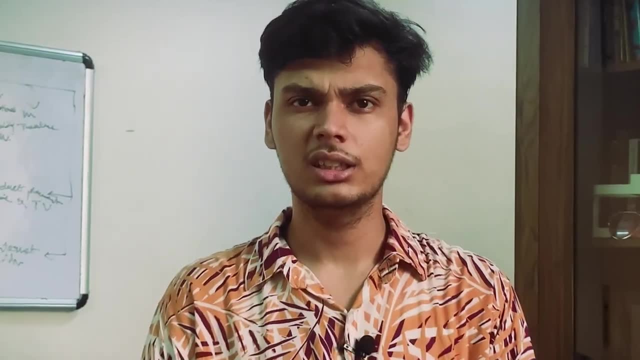 even have a wavelength, look very similar. Think of it this way: For a colorblind person, red and green might look very similar Doesn't mean that there is no difference between red and green. it just means that that person is not capable of perceiving it. 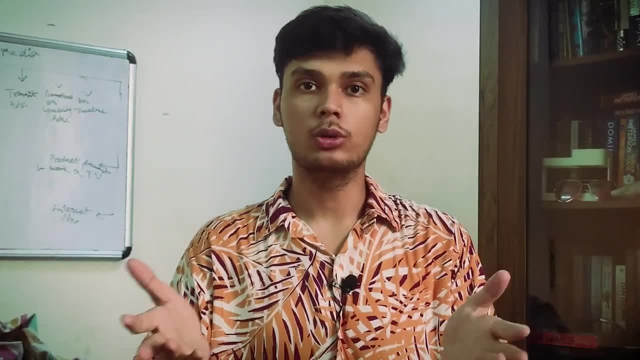 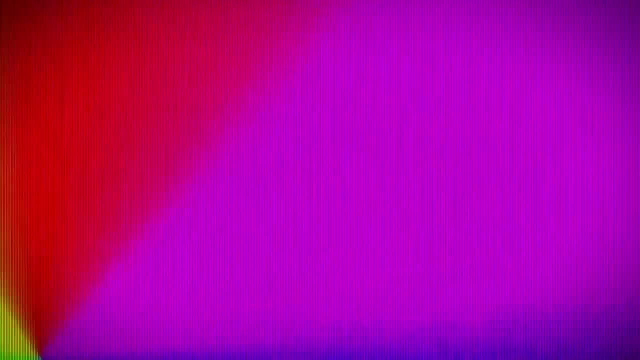 Even though red and blue don't meet on the electromagnetic spectrum doesn't mean we can't flash these colors simultaneously in front of our eyes, like we do red and green to make to fake yellow. It is this process that creates this entire part of the color wheel.